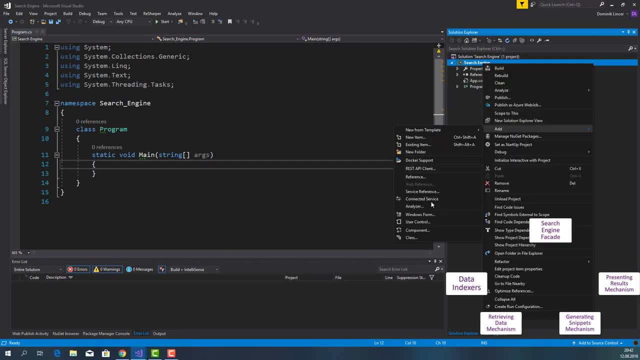 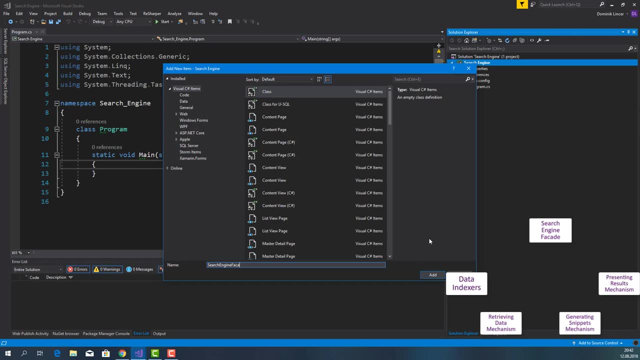 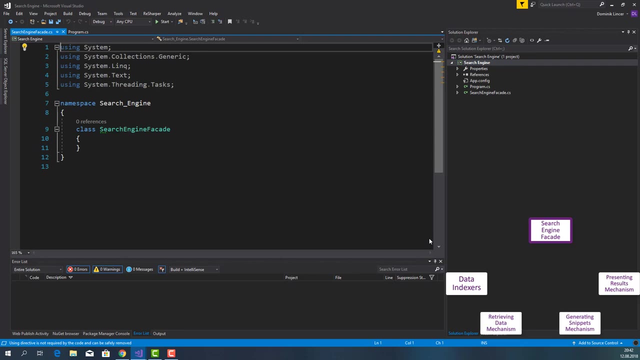 So let's quickly implement our first class, The search engine facet. Okay, now, when you've got that, We actually don't need it at this time. We will leave it as it is. You later came to it back. Maybe let's call it just public for now. 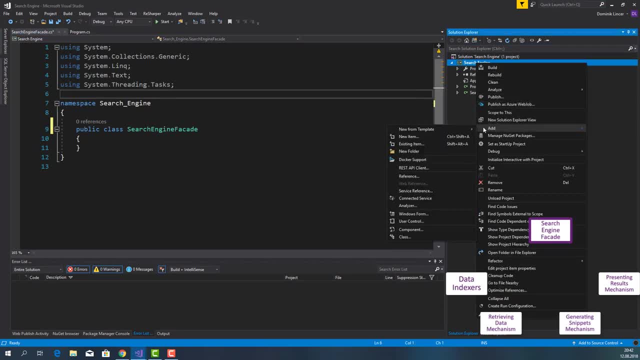 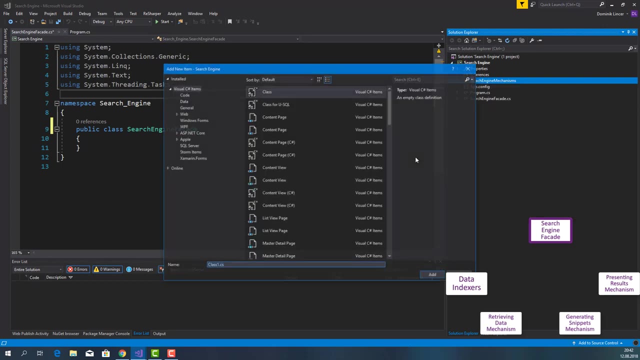 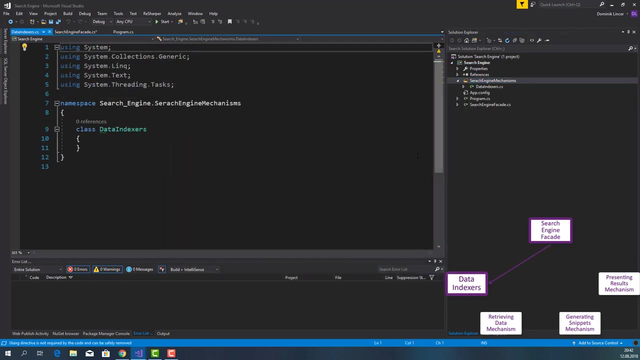 And let's jump to creating the first folder: search engine mechanisms. And let's create our first mechanism. that will be data indexers. Data indexers Are used to get the information where the web pages are stored with which indexes. So, for example, when user types a query to a search engine, it will say that the results are stored in index five, seven and so on. 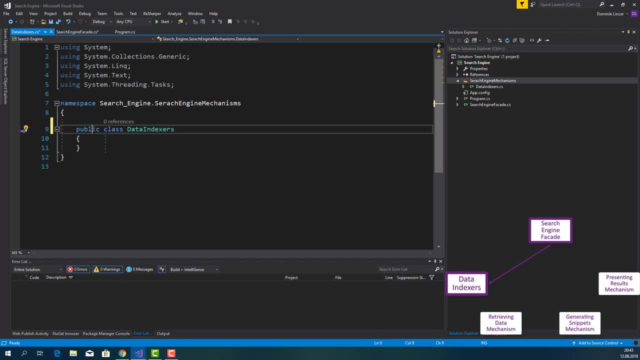 So let's implement that. Call it public, Create our first method. It will be type of integer array And It will be called get indexes of stored data. It will take a string as a parameter, called query, And this method will write on the console. 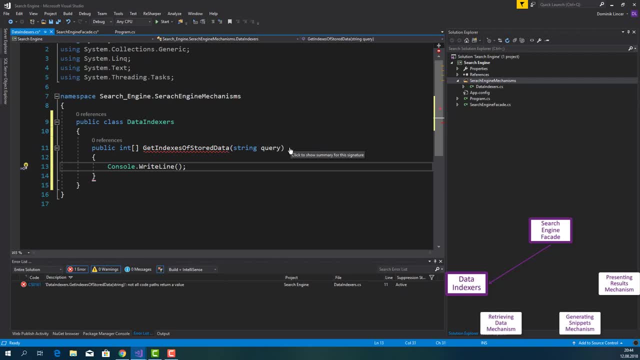 To user A string starting with Our query, And query can be found At indexes. Let's say one first index, five And eight, And we'll also return A new array With the same indexes And eight. So that's all for this class. 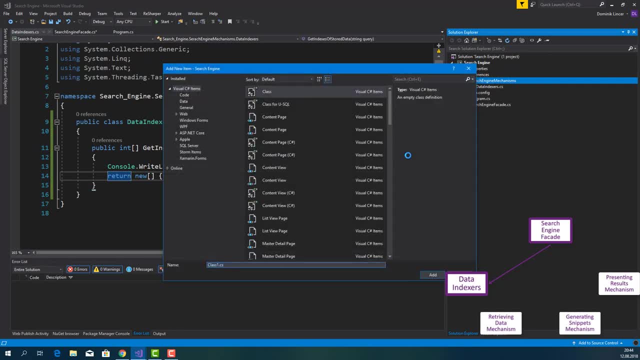 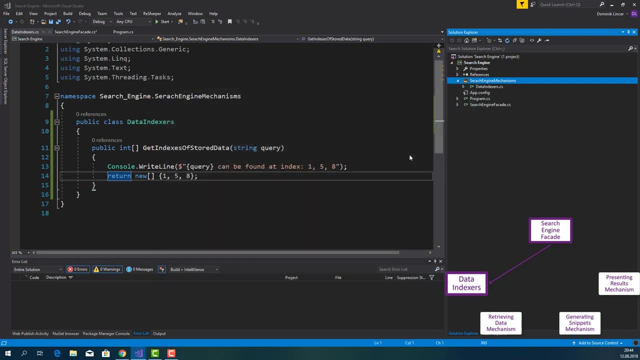 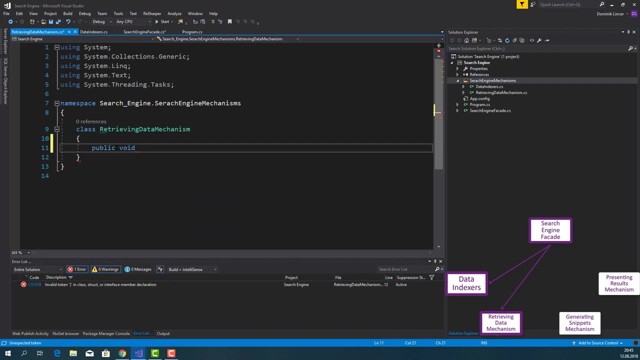 Let's create the second one And it will be called retrieving Data mechanism And it will have also one method That will be called, Will be type of void And will be called Get data With Our Array of indexes. 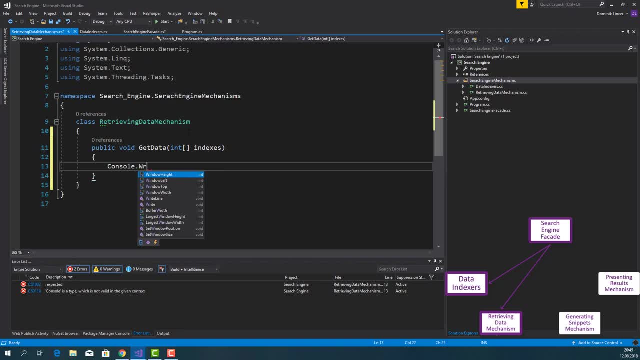 And at the beginning We are going to write To user Downloading Web pages with indexes. Let's make a colon here And Iterate Through With For each loop Through Our collection Of indexes With. 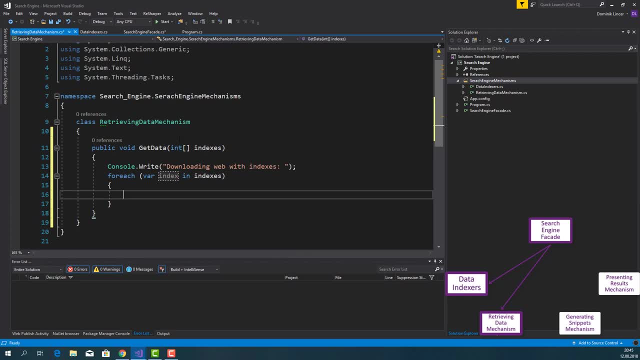 Every index And also Write This index, Console Write Index With Empty space, Here Also with colon To make it look better, And now only Call the console Write line Method, And Now only. 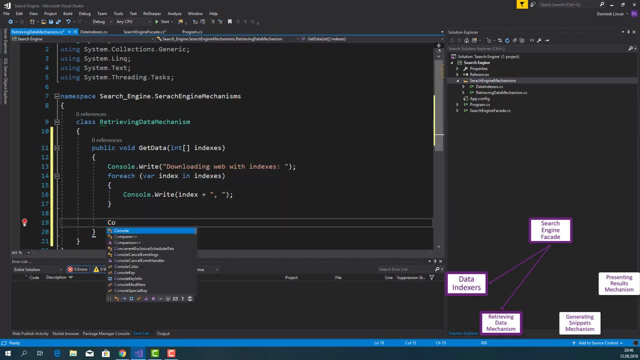 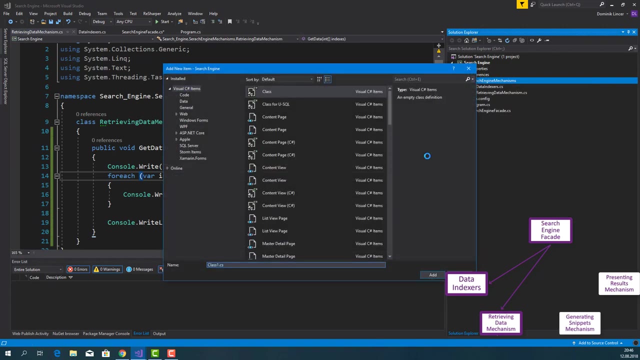 Call the console Write line Method To Jump To the next line, To not make Too many lines, Too many Text In one line. And now Our First Class, Third Class, That is called: 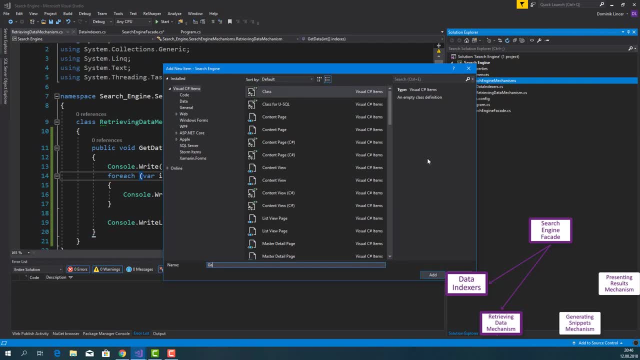 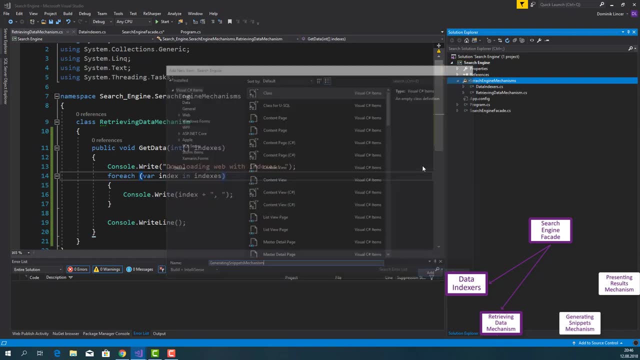 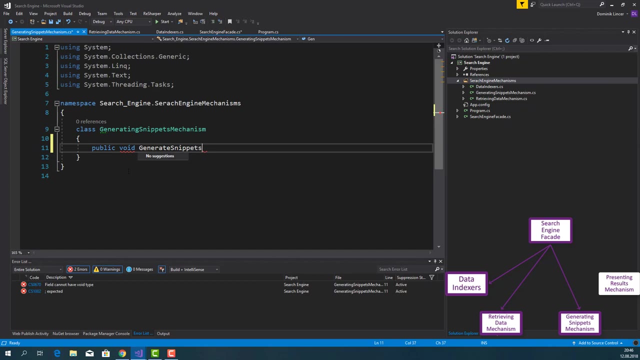 Generating Snippets Mechanism. This class Will have Method: Generate Snippets Method- Generate Snippets Method- Generate Snippets Method. And In This Method We Will Write: 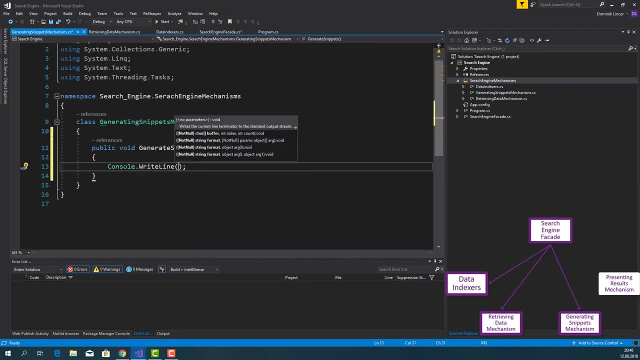 To User This Action That Is Actually Doing. We Are Actually Creating Snippet With Most Important Informations From Page, Because We Don't Want Different. 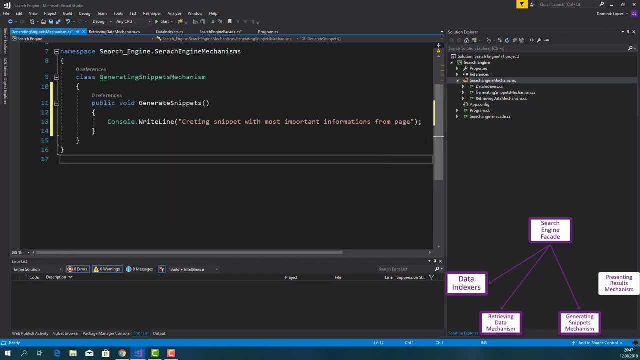 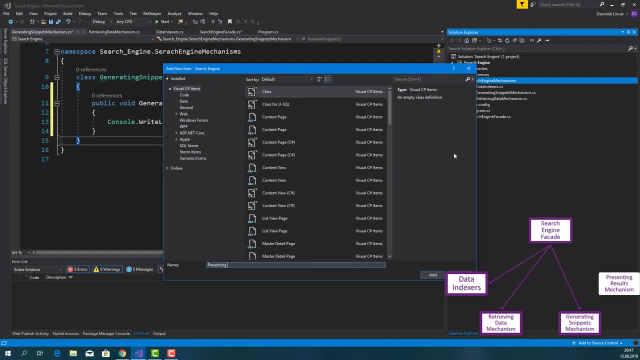 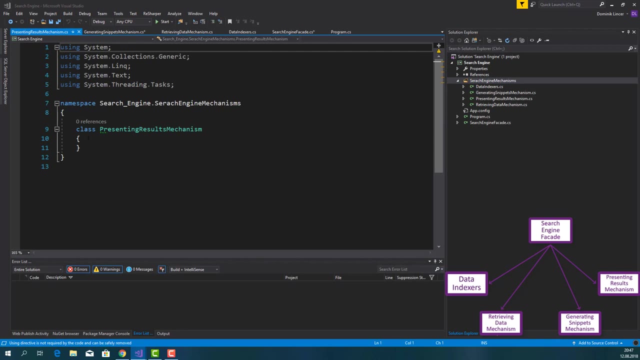 Informations In A Nice Way, So To Present It In The Best Possible Way. We Will Also Need A Presenting Results Mechanism And In 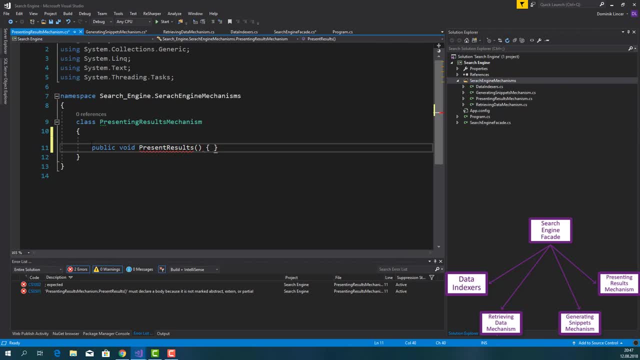 This Mechanism We Will Print To User, Presenting Data In A Good Looking Way. Let Me Quickly Check If I Called Each Of These Classes. 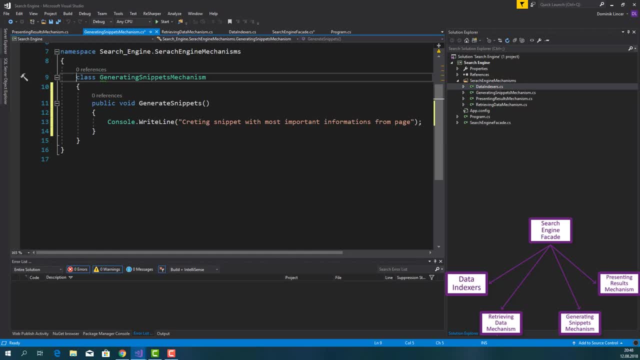 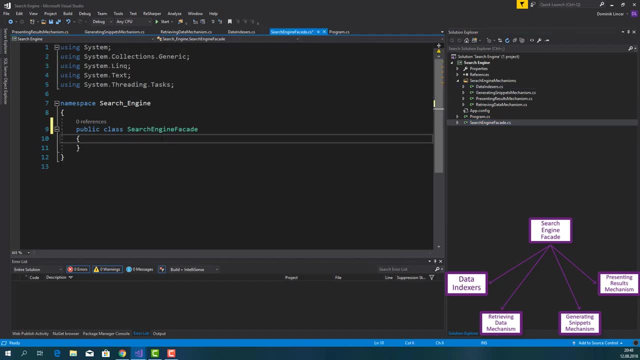 Public- This One, We Generating Snippets Also- And Data Indexers Have That, So We Can Go Back To Our Search Engine Facade And Make 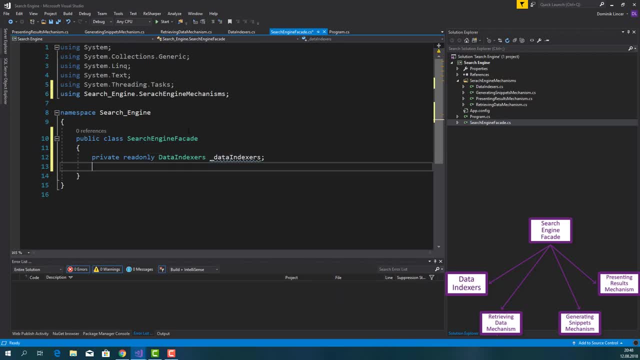 Fields For Each Of Our Mechanisms, Starting With Our Classes: Retrieving Data Mechanism, The Third One From Our Classes Generating Snippets Mechanism. And 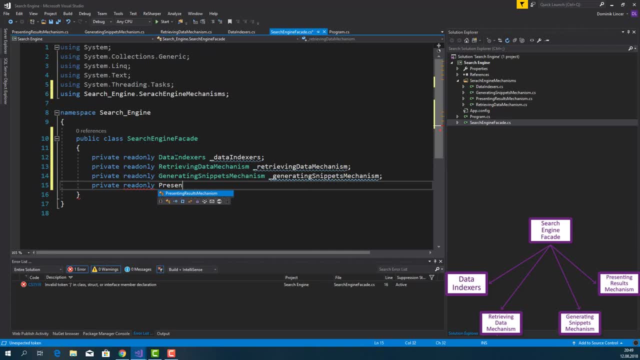 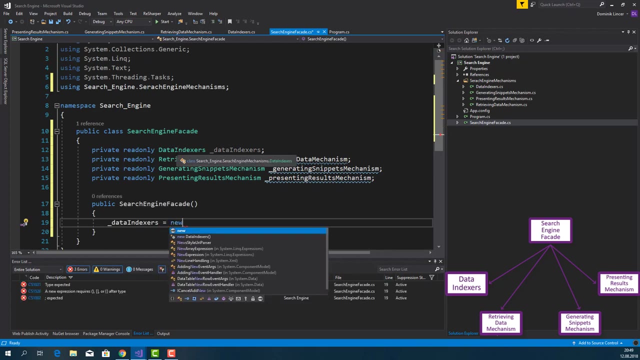 The Last One, Presenting Results Mechanism, And We've Got All Of Them, So Now We Can Call The Constructor In Which We Are Going. 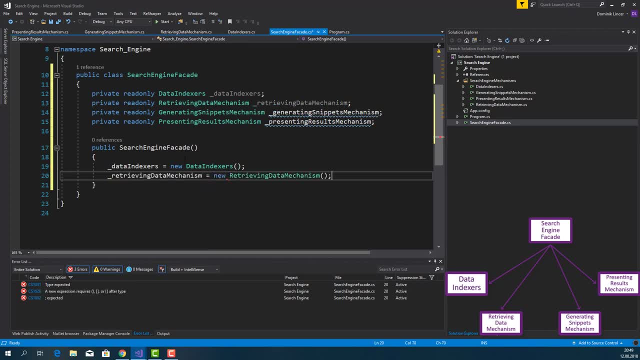 To Insanitate, If Each Of These Classes, The Data Indexers To This Presenting Results Class, And Now, When You've Got That, We Can. 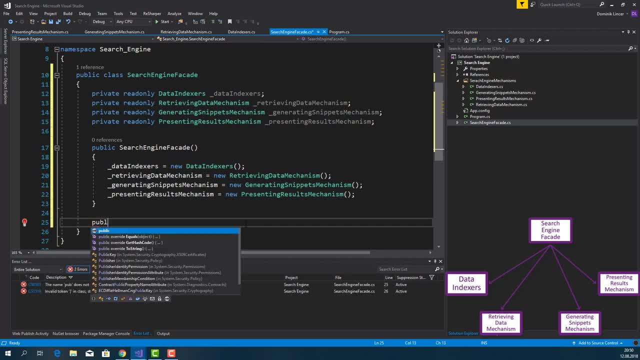 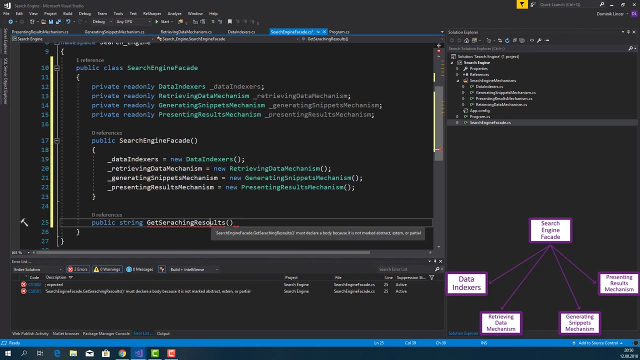 Go To Create The Method For Searching The Results. It Will Be, It Will Return As A Query Without This Letter And We'll Take A. 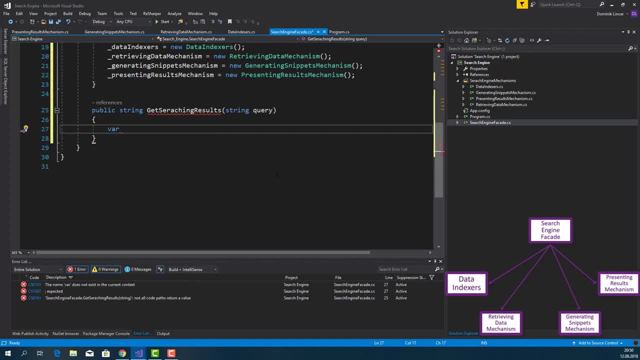 Query As A Parameter, So Let's Create A Variable Called Indexes, And It Will Be Equal To Data Indexers Get Indexes, So Let's. 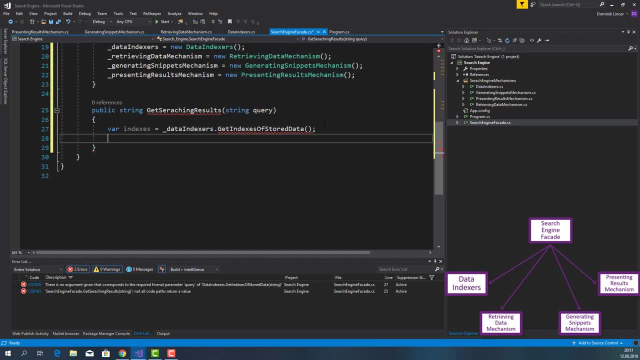 Call It Now With The Query As A Parameter. Now We Can Use The Retrieving Data Mechanism Class And Use The Get Data For The. 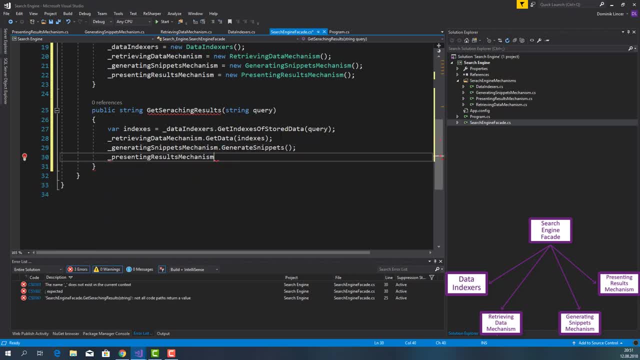 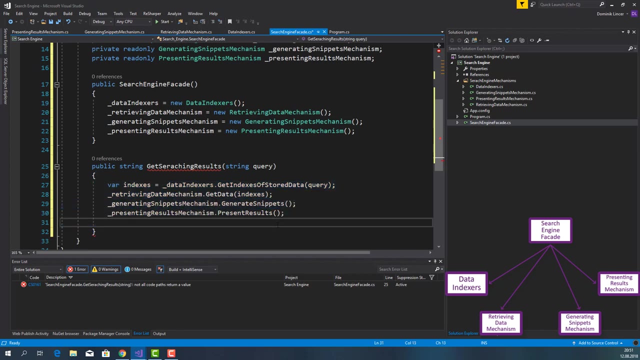 Indexes That, The Presenting Results Mechanism, Present Results. And Now We've Got Everything In Just One Method, In One Class: The Get Searching Results. 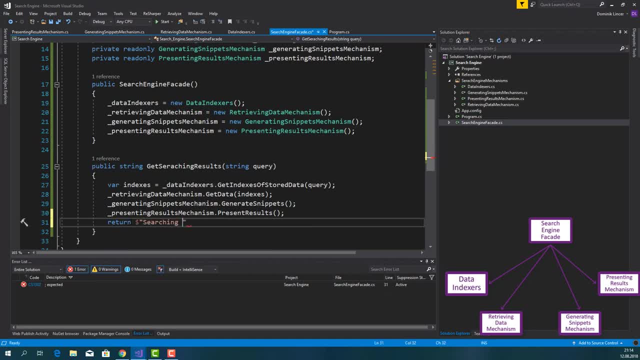 Will Do Everything That We Need To Get Data And Our Query That User Has Typed And Here Will Be Our Results. But It Is Only 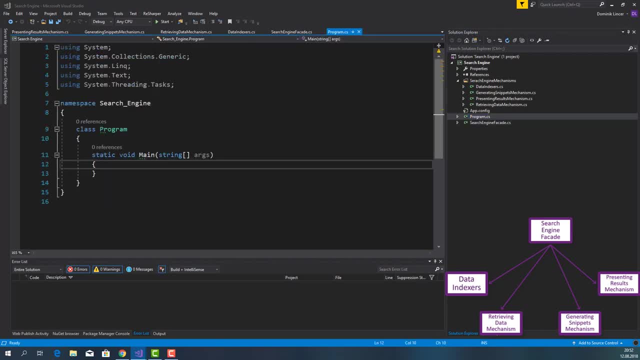 A Mockup Of An Application, And Now Let's Use It In Searching. Search Engine Facade Is Equal To A New Object, And Now Let's. 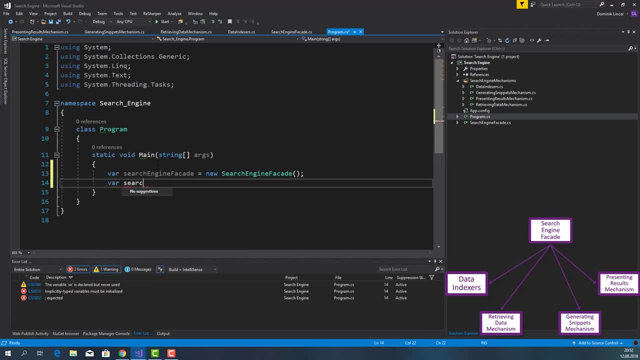 Get Our Results. Create A Variable For That. Searching Results Is Equal To Search Engine. Facade Query For Example. My Query For That And We: 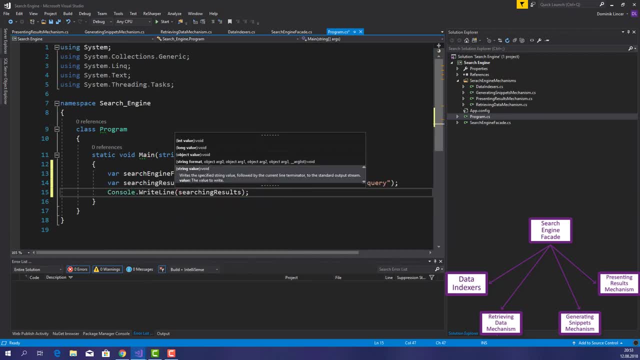 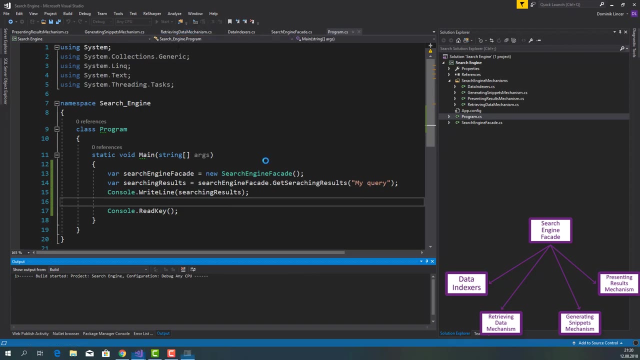 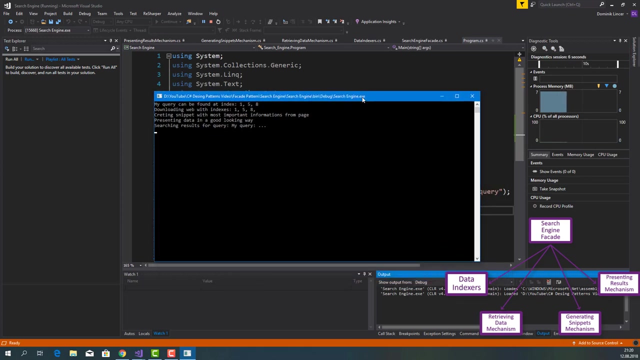 Can Print It To The Console Window. This Results And At The End Called The Read Key Method To Prevent Our Process. So As You Can, 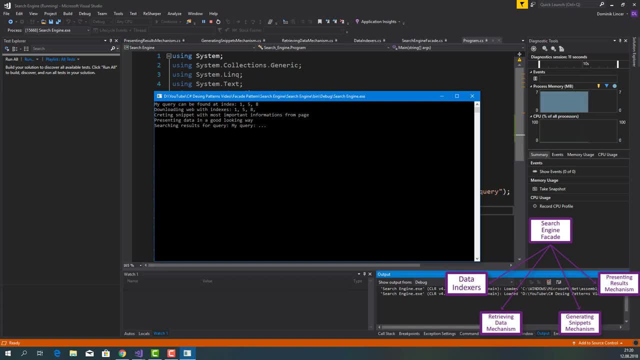 See, We've Got Our Process In These Five Steps. My Query Can Be Found At Indexes. We Then Will Download The Web Pages With Google. And A Link In The Box You Can Print It. To Print It At The End, The End Of Our Process, To Prevent Our Process. Print. Can Be Found.